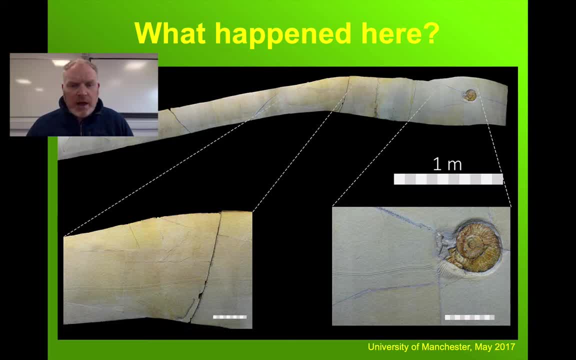 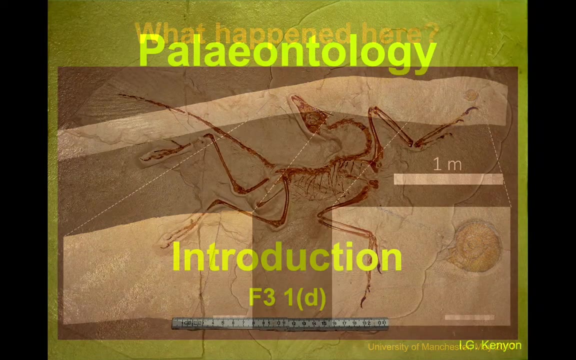 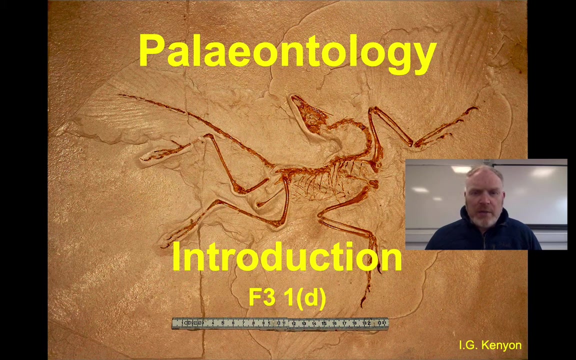 as it's been dragged, perhaps by a current, along the seabed before the animal itself finally dies and becomes incorporated into the sediment. It shows, perhaps, that fossils give us huge amounts of information about environments, about time, about evolution, about plate tectonics. 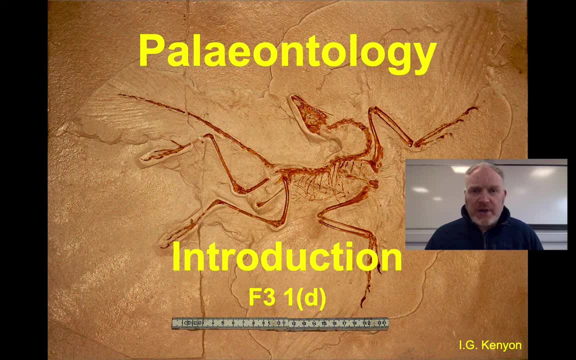 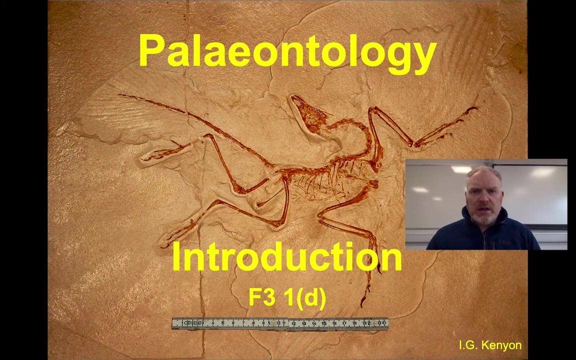 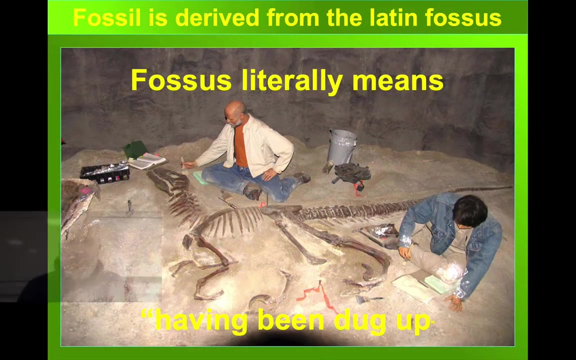 about all sorts of different aspects of how the Earth works, All rolled together in this sub-subject within geology we call paleontology. So let's have a look at what we actually are talking about when we're looking at fossils. Fossil comes from a Latin word. 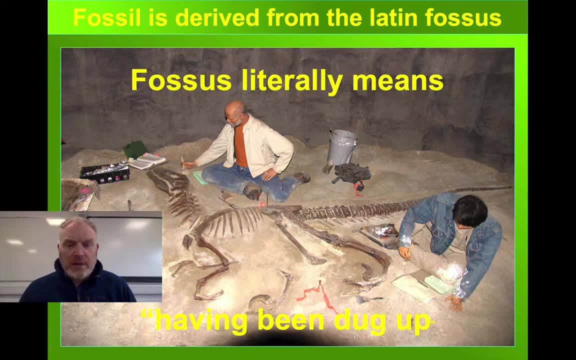 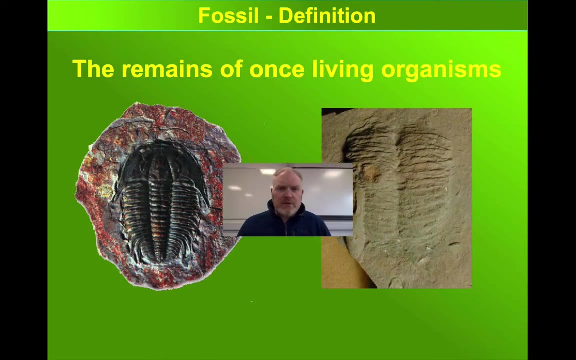 the word fossus, And that means literally having been dug up. A fossae, for example, is a ditch. in Latin, A fossil itself is defined as the remains of a once-living organism Or some evidence of their activity. 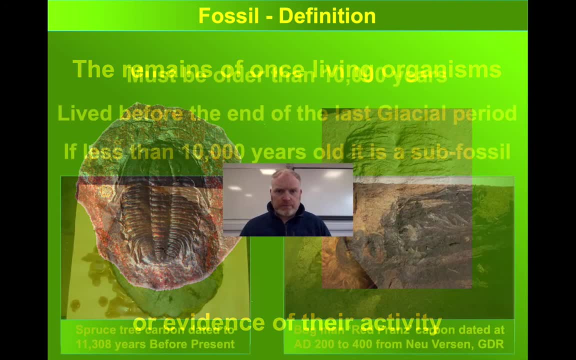 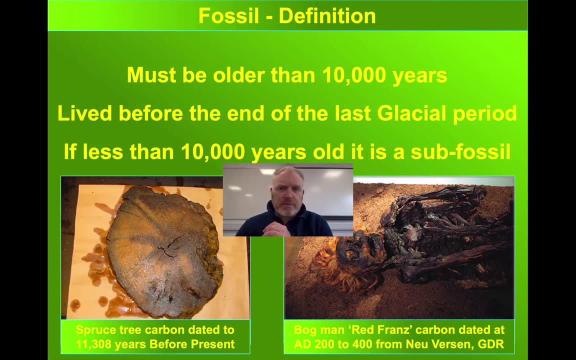 Let's have a look at breaking that down a little bit Now. there is a definition that we add to that, which says that to be a fossil, it must be more than 10,000 years old, Or to put it another way, to have lived before the end of the last glacial period. 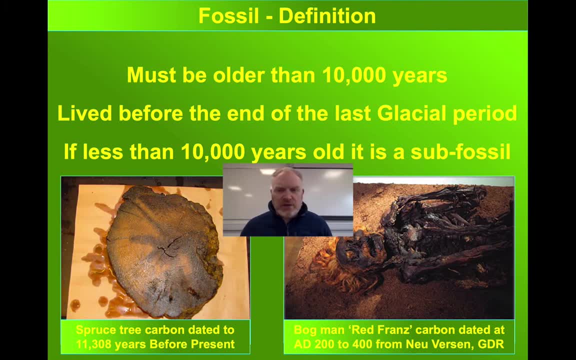 the last ice age. Less than that, we talk about a sub-fossil. Now, perhaps it's just because I'm a quaternary geologist myself, I'm perhaps less hung up on this definition than other people. For me, it's more about the evidence of past life. 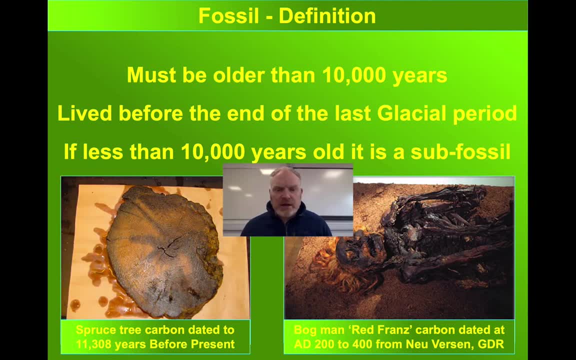 and past activity that really are key to making it a fossil. The distinction between these two examples of a spruce tree that's dated to just over 11,000 years ago and a human fossil from a peat bog, which is what, 1,800 years old, maybe, 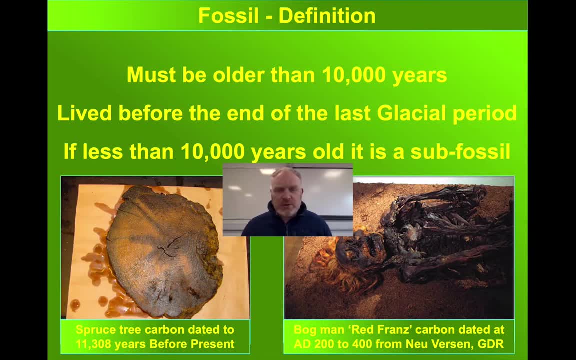 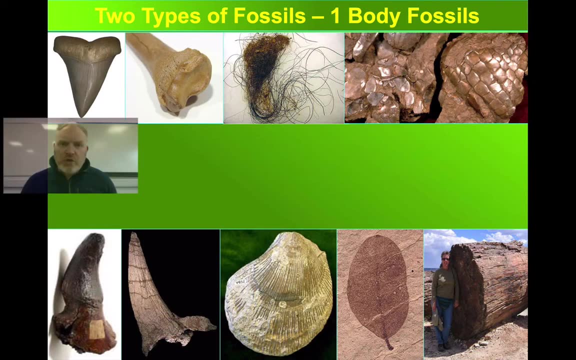 I don't see the massive distinction between them, And it's certainly not one we should worry about. There are two types of fossils that we need to deal with, perhaps slightly differently. The first of these is a body fossil. Now, a body fossil is some part of an organism's anatomy. 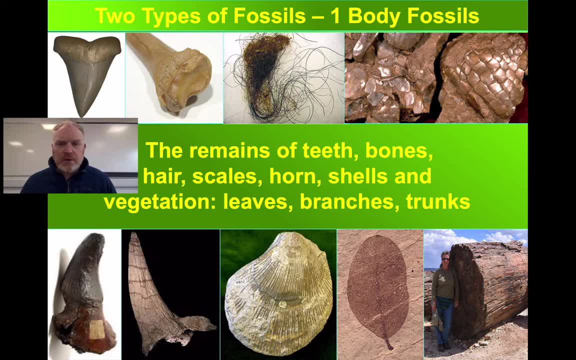 that's been preserved in the rocks. Now, typically these are things like teeth, bones, shells, horns. in plants it could be leaves or branches or roots or trunks of trees- Some part of an organism's body that gets preserved. Now it could be preserved as an imprint of that. 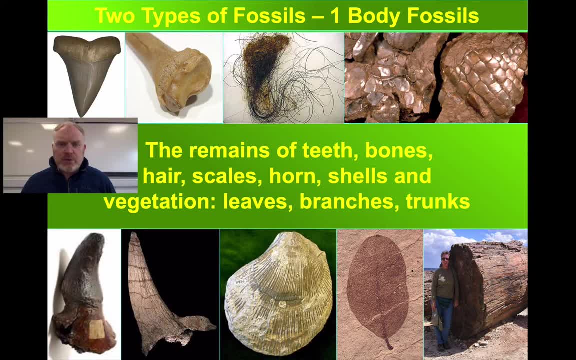 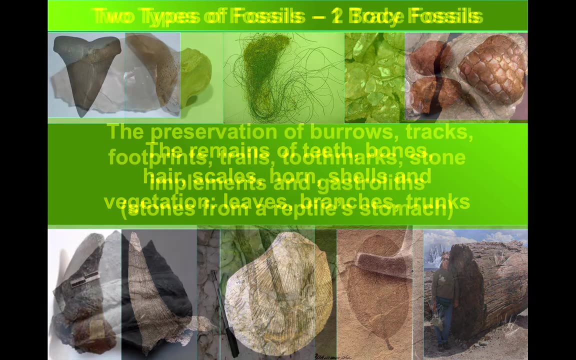 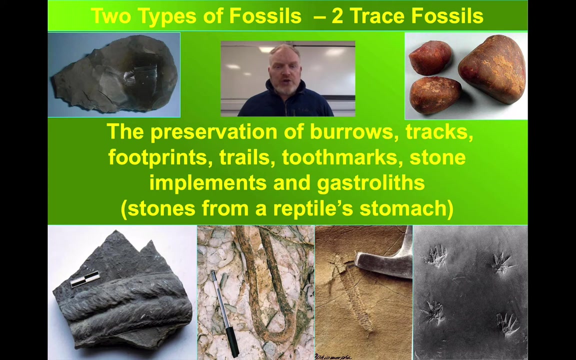 but it's the body itself that we see a record of within the rock. Most of the fossils we deal with are body fossils, But they're not the only type. We also see a group of fossils we call trace fossils. Now, a trace fossil is a record of an organism's activity. 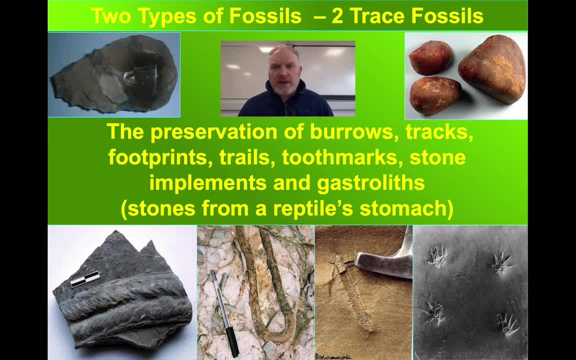 An imprint it left as it lived Now. there's a huge range of these. I've listed some of them here, But they are perhaps the best known. We can also include things like teeth marks For human fossils. stone implements are an important piece of evidence. 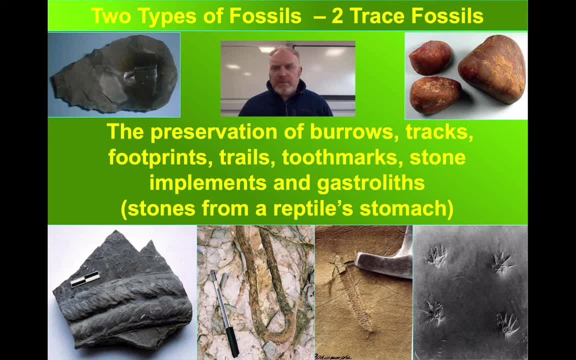 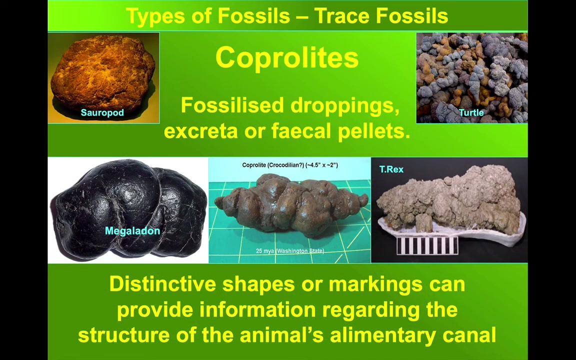 Even gastroliths, The stones that dinosaurs ate to help them grind up their food. All of these are fossils, and these again can give us some crucial bits of evidence about past life. some of the more famous examples of this include things like coprolites. these are: 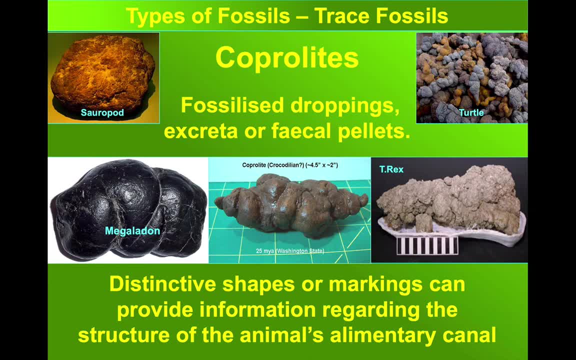 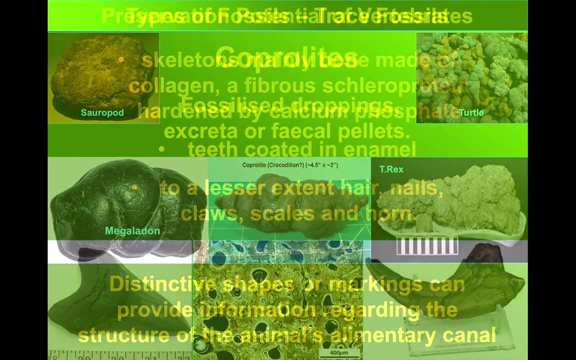 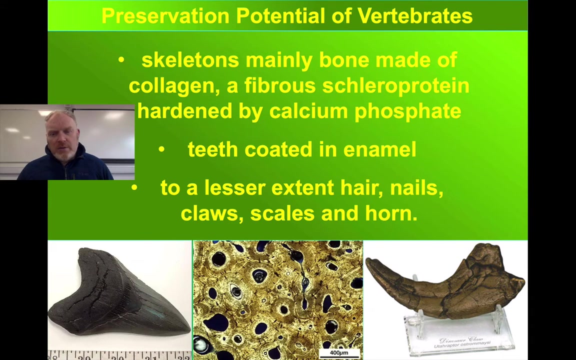 fossilized dung feces preserved in the rocks. you can see there's a whole range of these things, um ones that give uh useful information about an animal's diet or um how it actually digested its food. now, different types of fossils are preserved in different ways, depending on what their body is. 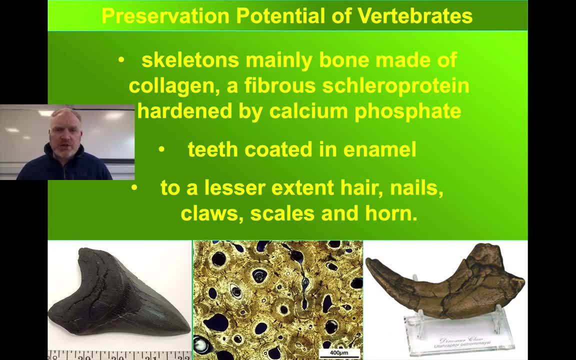 made from. it's an idea we call preservation potential. we'll talk more about this in another lesson, but where we see organisms that have hard parts- so things like skeletal buttons, uh, in a vertebra or teeth, okay- are most likely to preserve, they're the most resistant. 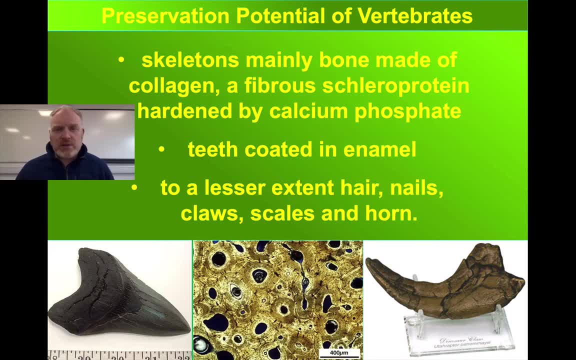 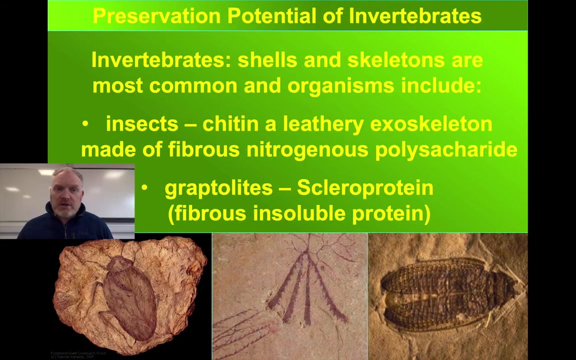 things to all the processes that can happen to an organism following or even during death. to a lesser extent, you can get other things preserved in more exceptional circumstances: hair and skin, imprints, horn, that type of thing for invertebrates. these are animals without backbones. um, these are perhaps the most common uh fossils that we find, and there are particular bits of 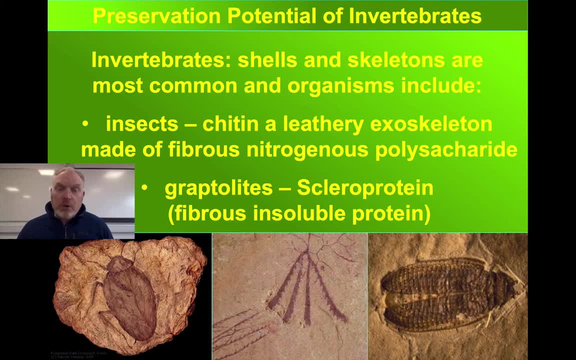 fossils that are more likely to preserve. so insects, for example, an incredibly common, incredibly diverse group um their exoskeleton is made of a material called chitin. um now, chitin is is relatively robust, particularly if there's no oxygen around. it does tend to break down in uh in uh aerobic environments. 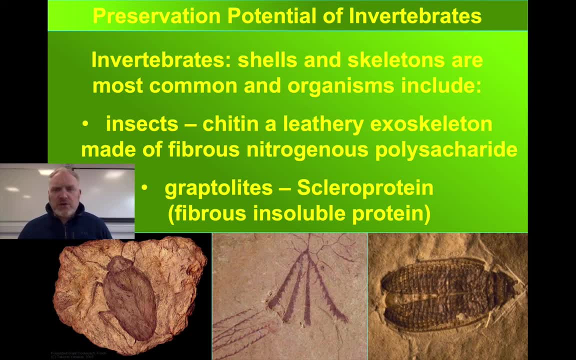 uh graptolites, a group of fossils that we're going to be looking at in for dating their um. their bodies are made of a uh called a scleroprotein, which is a bit like fingernail material now that can preserve again, predominantly in anaerobic environments. 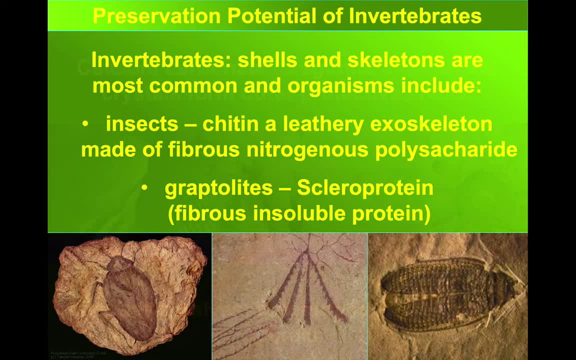 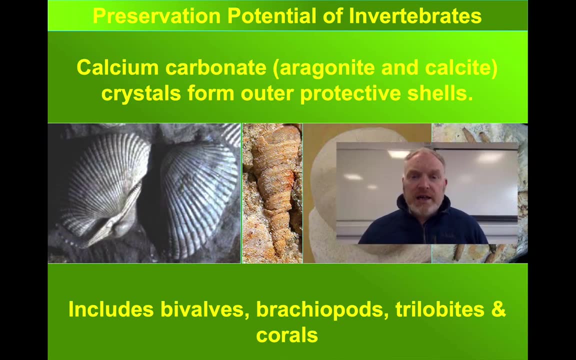 but the most common preservation we see for invertebrates is in the shells- shelled organisms- small invertebrates with these hard shells- are most likely to preserve and they're the most frequent um fossils that we look at in our course. uh, usually a calcium carbonate, either calcite or a slightly different form of calcite called aragonite. 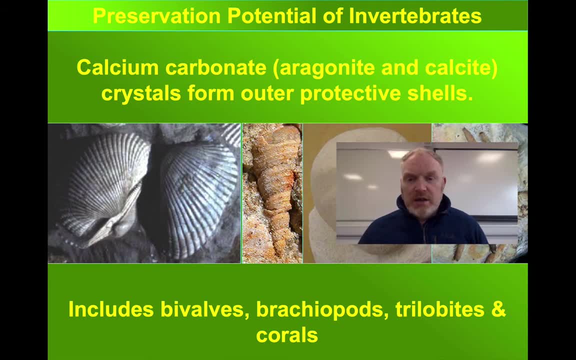 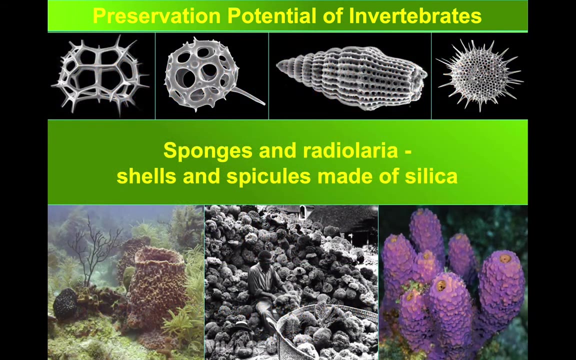 um form, this hard outer shell that stands a reasonably good chance of being preserved. so bivalves, brachypods, trilobites, corals- all have this type of structure. less commonly, we do see some um invertebrates that have a shell or a skeleton made of silica, uh sponges or uh microfossils called radiolera. 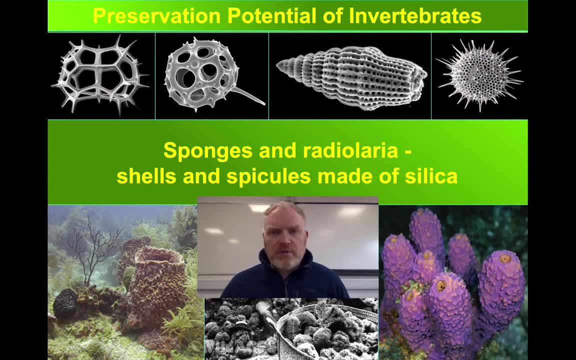 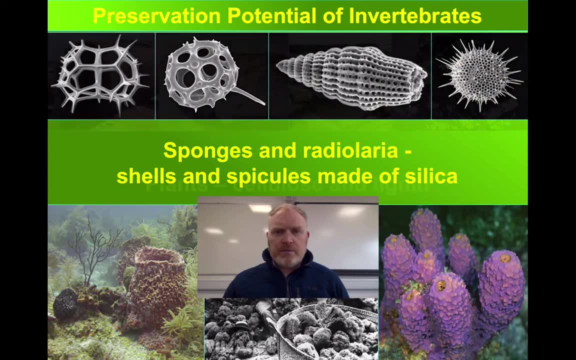 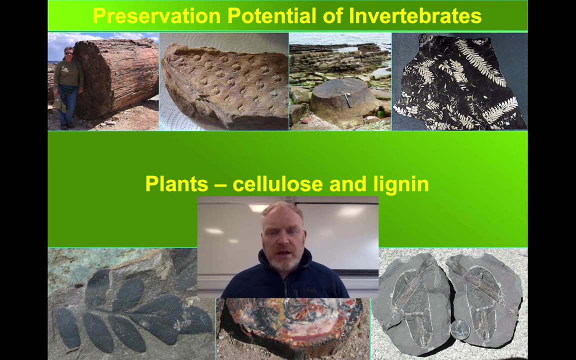 uh, we don't um really study these in in too much depth, but you know they do exist and they do preserve plants too. um will preserve in particular, uh, cellulose or lignin, which is sort of the woody part of the cellulose, which is the woody part of the cellulose, which is the woody part of the. 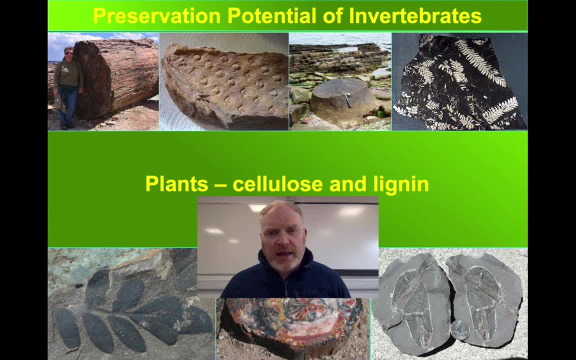 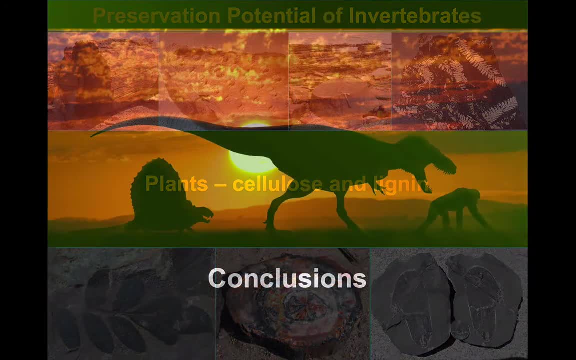 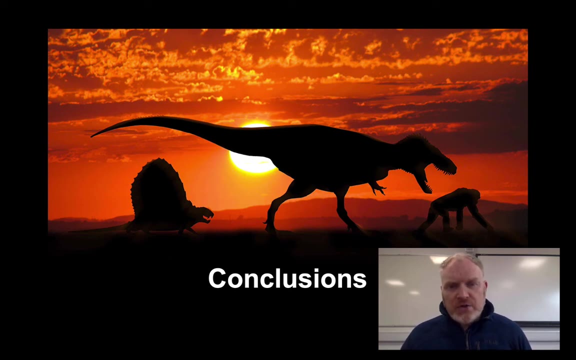 of trees and plants that can preserve, in particular, environments. so, to conclude, fossils give us a huge amount of information that supplements what we find already within the rocks about the age of those rocks, the environment in which they were deposited, the conditions that existed on Earth. 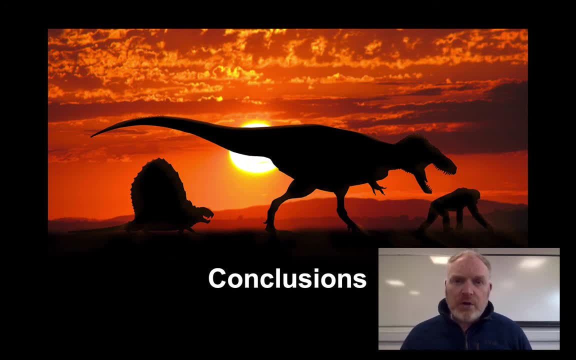 and also the history of life on Earth, how life has evolved in response to changing geological situations. For us as geologists, it's really important that we understand what the fossils are telling us, So we need to understand more about the fossil record. 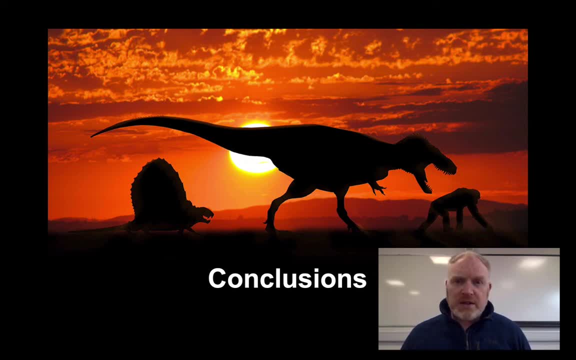 But that's for another lesson. I'll see you then.